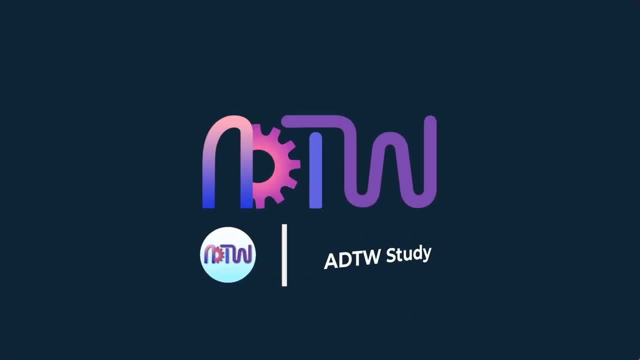 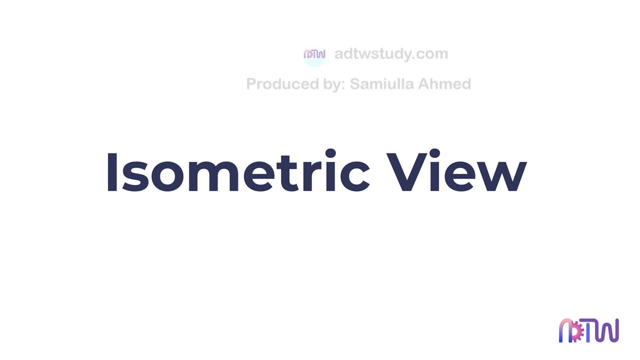 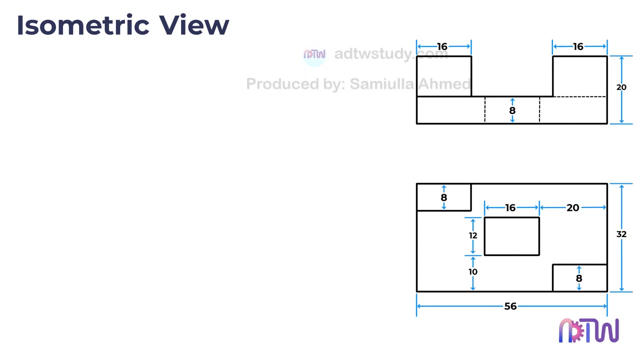 Isometric view. In this video we will learn how to construct an isometric view using orthographic projections. This is our 8th video on the topic. These are the orthographic projection of the object. To construct the isometric view or 3D view of the object, we first need to create the 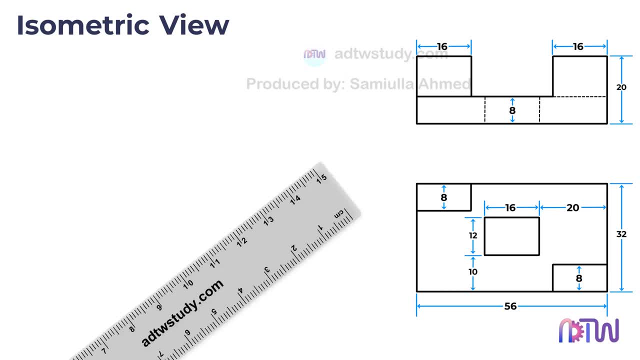 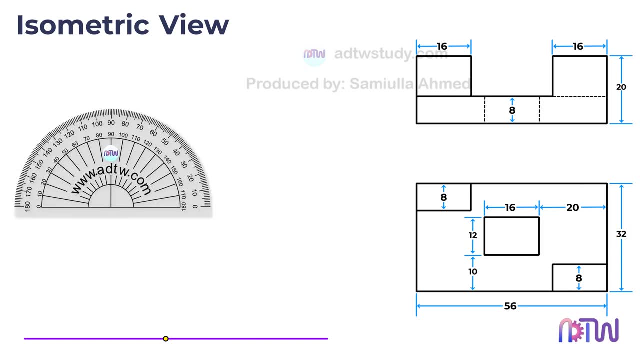 isometric axis. To do this, take a ruler and draw a horizontal line. Then mark a center point on this line. Next, take a protractor and mark 30 degrees on both sides of the center point, as well as 90 degrees. Draw lines passing through these points from the center point. 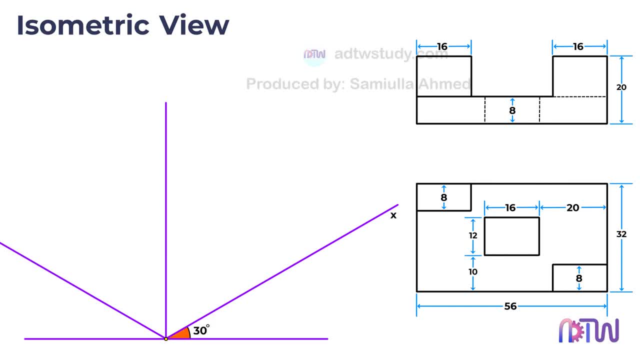 The line passing through the 30 degree mark will be the x-axis, the line passing through the 90 degree mark will be the y-axis and the remaining line will be the z-axis. With these three isometric axes in place, we can now construct the isometric view. 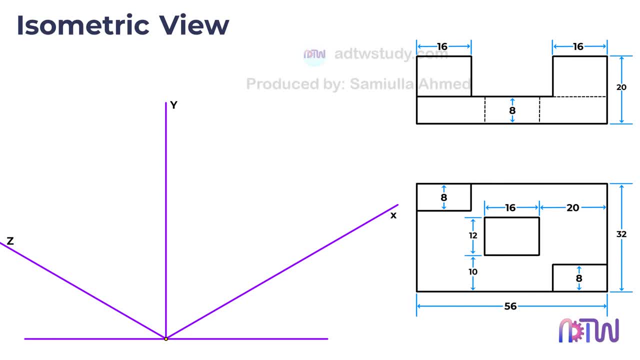 Next we need to decide whether to draw the front view in the x-y plane or the y-z plane. It's important to remember that the front view should only be drawn in these two planes and never in the x-z plane. The top view of the object is always drawn in the x-z plane. 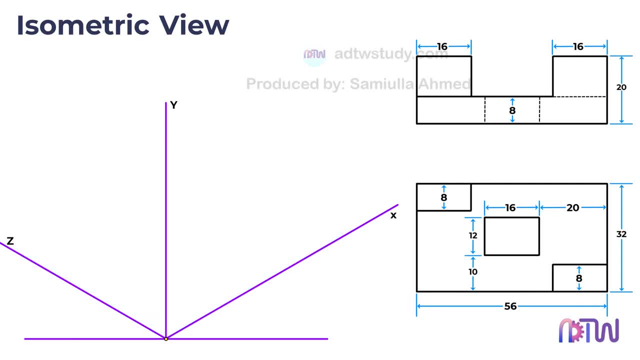 so that's another key point to keep in mind. In this video, we will be utilizing the first angle method to solve the problem. The figure on top is the front view and the figure on the bottom is the top view of the object. Let's start drawing. 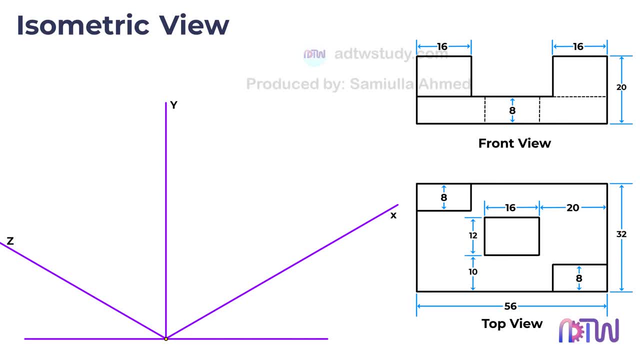 As usual, we'll begin by drawing the base of the figure. From the top view, we can observe that the length of the base is 56 millimeters and the width of the base is 32 millimeters. Take a drafter and draw the outline for the base, making it 56 millimeters in length and 32. 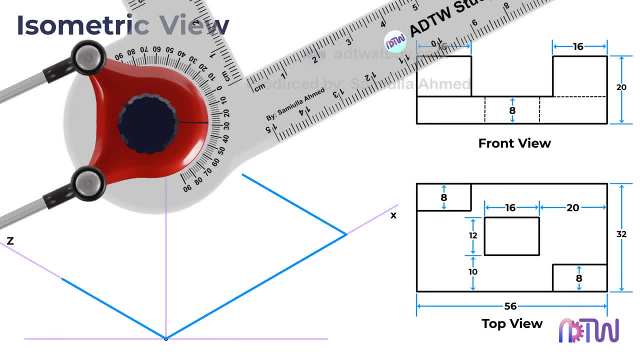 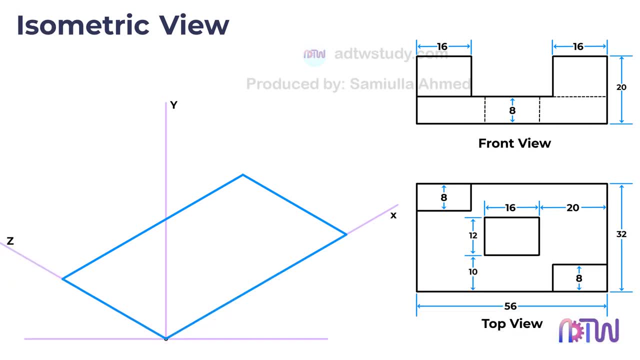 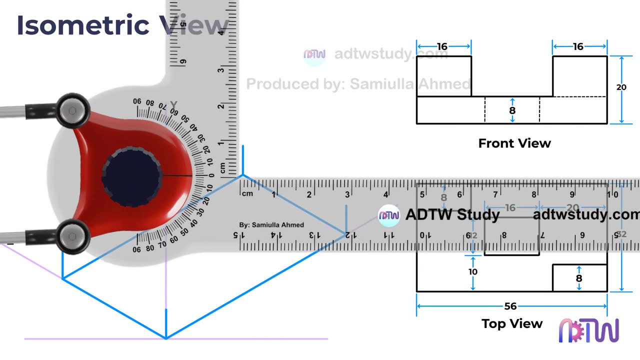 millimeters in width. Next, we notice that the thickness of this base is 8 millimeters. To represent this, extend the vertical lines by 8 millimeters from each corner point of the rectangle. Now join the endpoints of the vertical lines to complete the outline for the base. 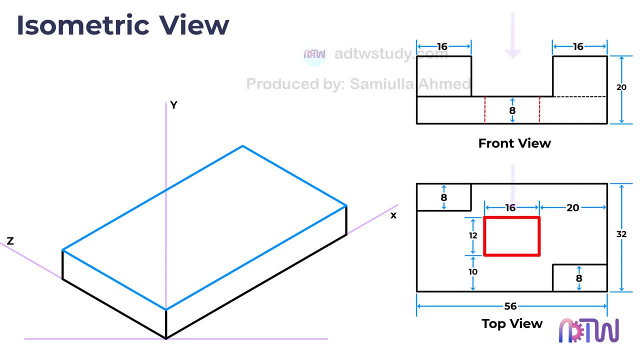 Moving on. there is a rectangular hole in the given object, As visible in the top view. the length of this hole is 16 millimeters and the width is 12 millimeters. This hole is positioned precisely in the middle of the base To locate the hole accurately. 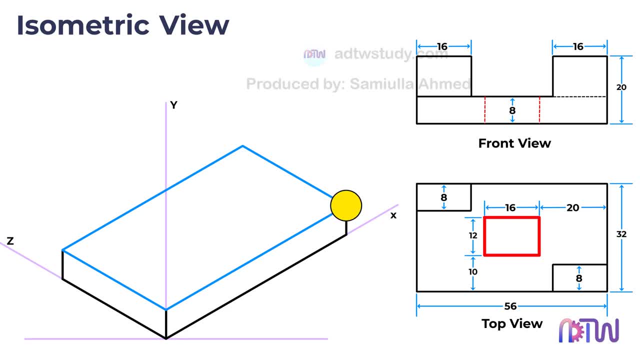 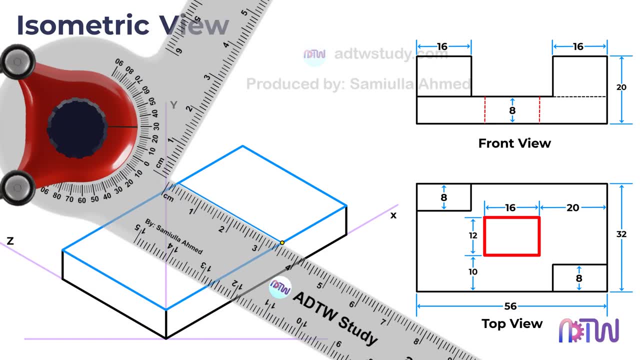 take a drafter and mark a point 20 millimeters away from this corner point. Draw a line parallel to the z-axis from this new point. Next, mark a point 10 millimeters away from the same corner point and draw a line parallel to the. 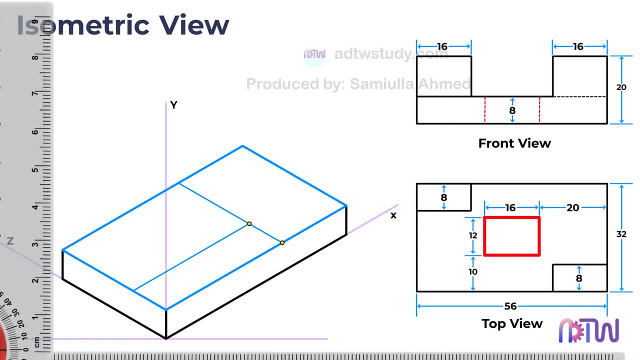 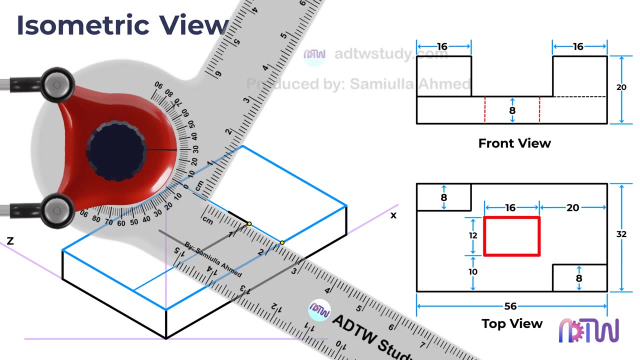 x-axis from this second point. These lines will serve as guides to help draw the rectangular hole at the exact center of the base. After completing the two vertical lines for the features, use them as references to draw a rectangle with a length of 16 mm and a width of 12 mm, representing the slot. 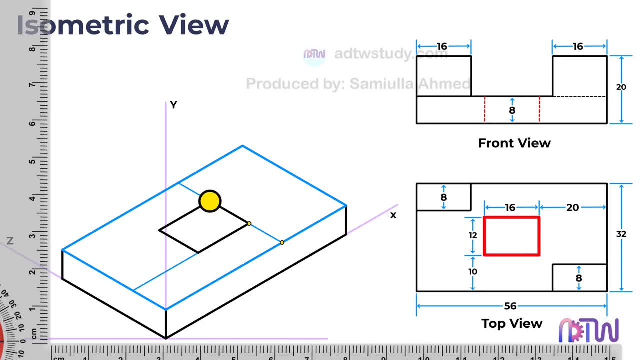 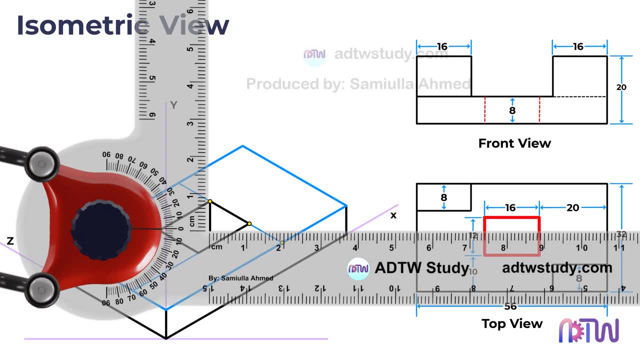 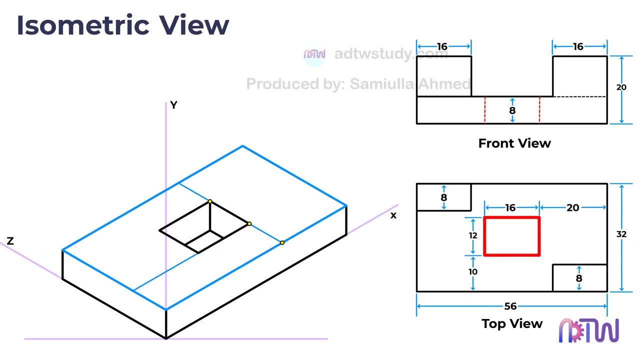 Extend an 8 mm vertical line from one corner of the rectangle to indicate the depth of the slot. Add the required detailing to the slot as per the design. Great, now that we've completed the base of the object, let's move on to drawing the two vertical features on it. 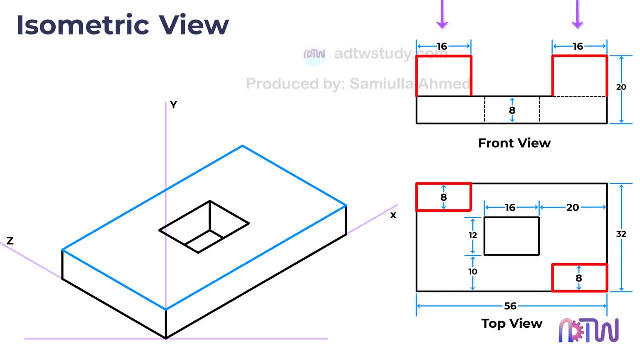 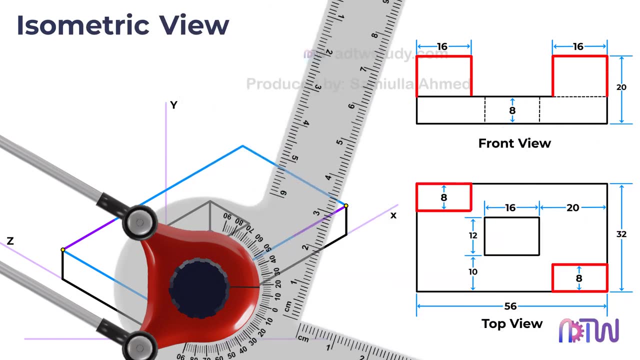 According to the front view, both of these features have a length of 16 mm, So take a drafter and mark points 16 mm away from the top corners of the base. Next, draw 8 mm lines parallel to the Z axis representing the width of the features. 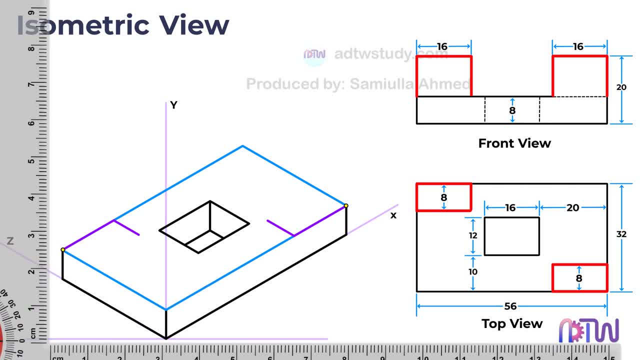 Now draw lines connecting the endpoints of the 8 mm lines to the edges of the base. These lines will complete the bases of the features. Next, let's focus on the height of these features. as seen in the front view, The height is calculated as 20 mm, which is the total height of the object minus 8 mm.